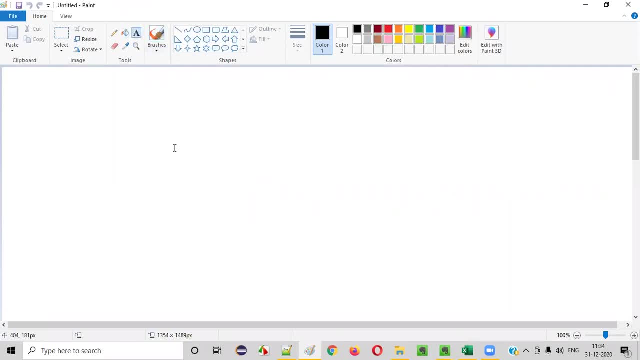 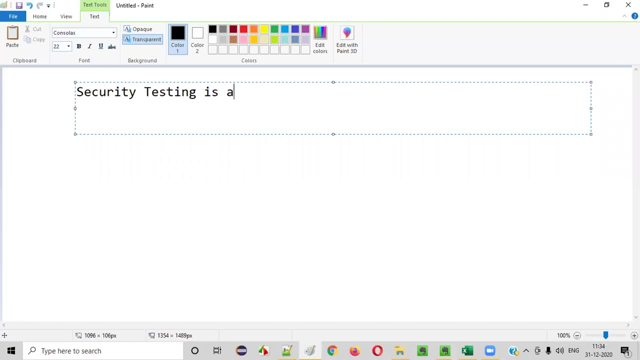 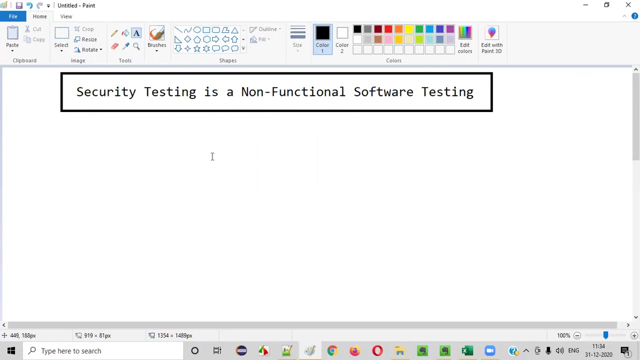 Before I explain what exactly is secure testing, let me first tell you that security testing is a non-functional software testing. So before I explain what exactly is secure testing, secure testing is a non-functional software testing. So when you categorize the different types of testings in software testing, 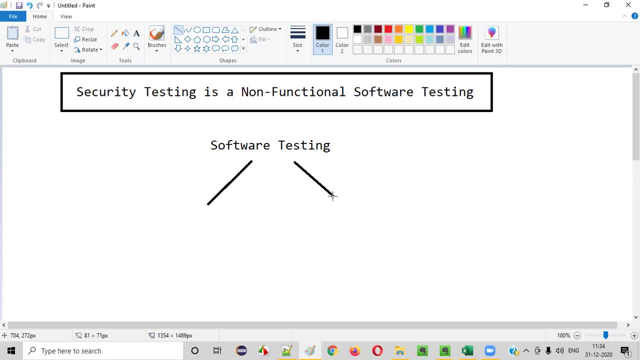 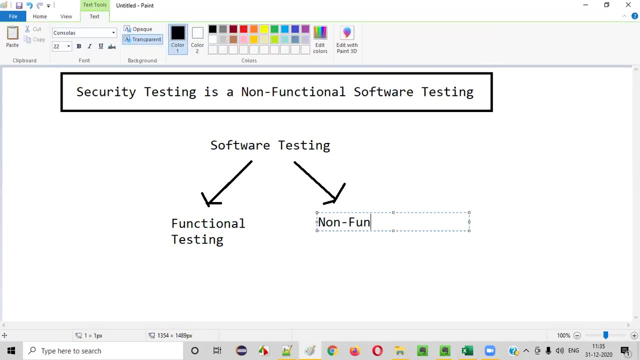 you can categorize the types of testing that you want to categorize. So you can categorize them at a high level into two types. One is functional, one is functional testing- types of software testing and other one is non-functional. Other one is non-functional testing type, category of software testing. 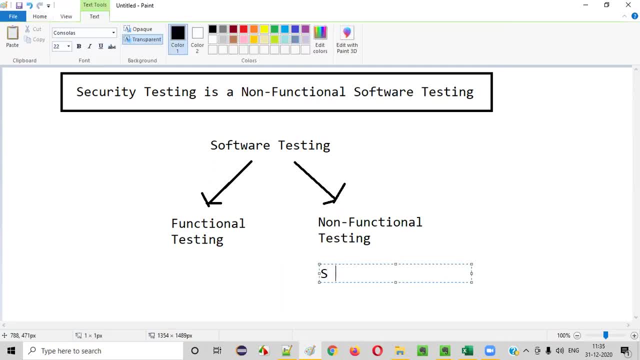 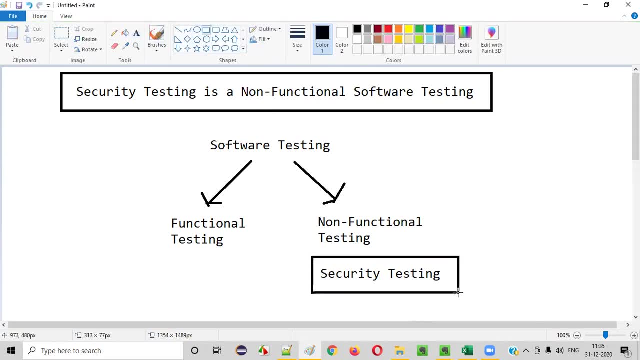 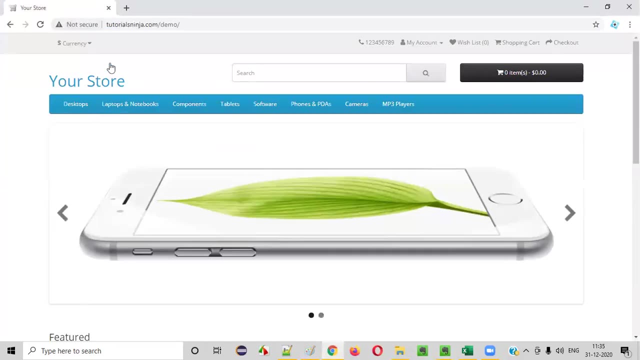 So this secure testing falls under the non-functional testing type. Security testing falls under the non-functional testing. That means as part of secure testing you don't have to test the functionality of the application In general software testing guys. as part of functional testing you will go to the application. 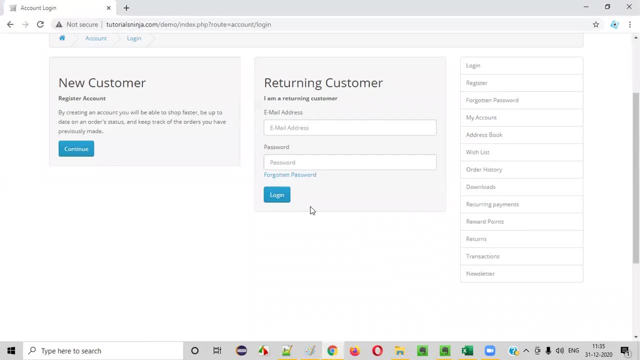 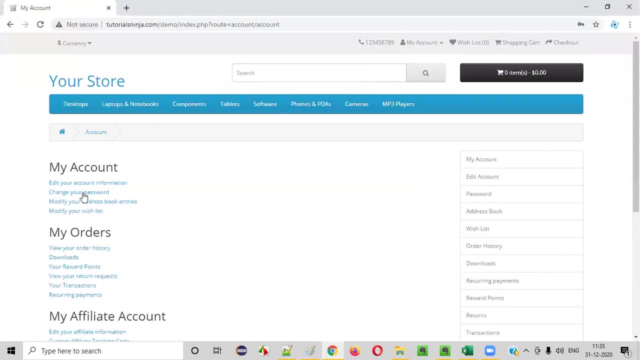 Let's say you have to verify this login functionality. Okay, let's say you have to test this login functionality. There you will provide the credentials and practically you will check whether the login functionality is working or not, really working or not. That comes into functional testing. 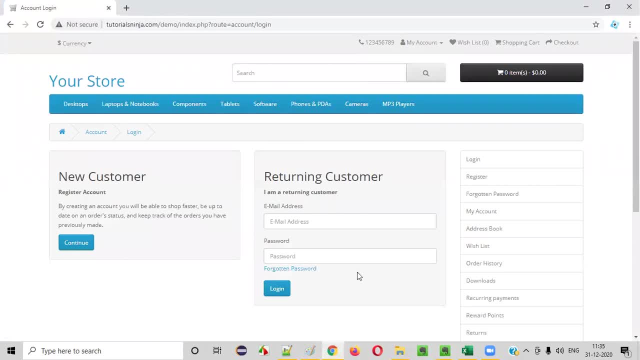 But in case of security testing, you don't have to test the functionality Of the application, guys. rather, we have to check what is the okay, how secure is this login functionality? Here, as part of secure testing, we are not going to test the functionality of the application. 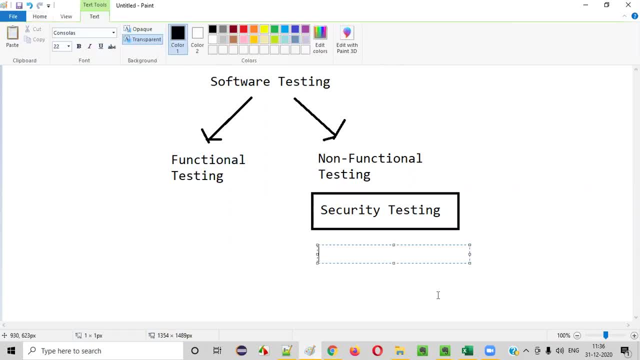 That's why we call it as non-functional testing. Here we'll test how secure is the application. How secure is the application? Okay, this is what will be tested as part of the secure testing. Now, without wasting any time, let's move to what exactly is secure testing. 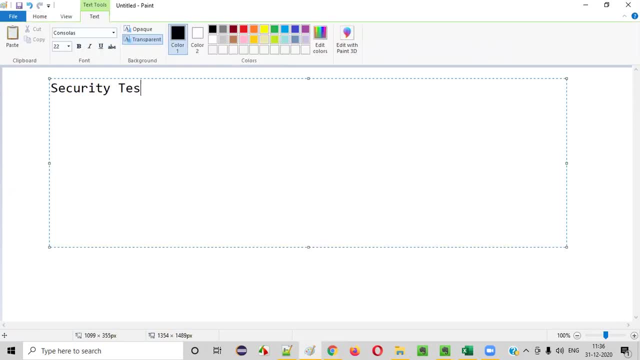 So what exactly is secure testing? Security testing is performed to- okay, let me write what exactly secure testing is. Later I will explain what exactly is secure testing. Secure testing is performed to identify- okay, or uncover whatever you call identify or uncover the security loopholes. 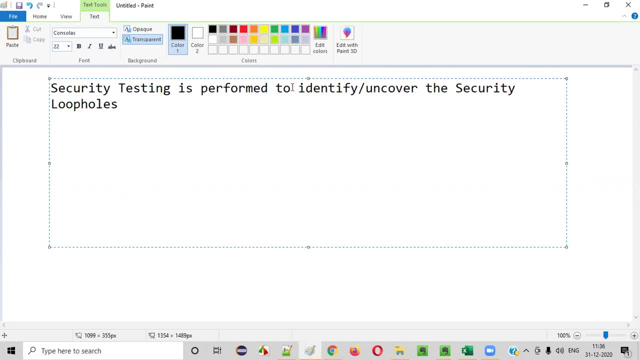 See, I just understand, guys, while I'm typing, Secure testing is performed to identify or uncover the security loopholes in the application and get them fixed. We need to get this security loopholes that are identified by us as part of secure testing in the application and get them fixed by the developers with an intention of with an intention of protecting the application. 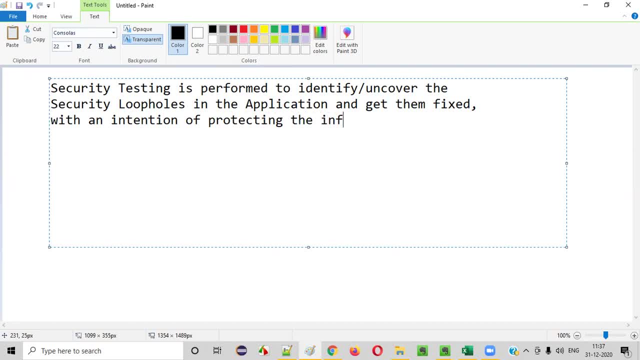 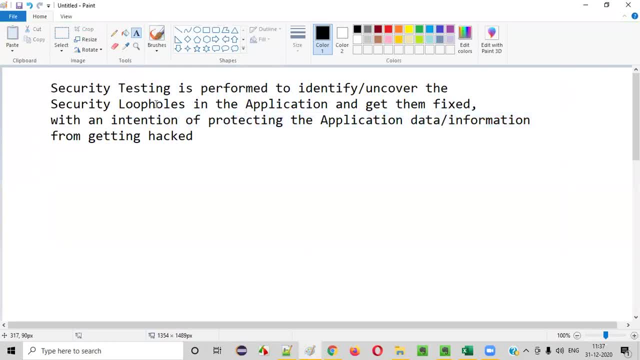 Okay, So this is what is secure testing is. If you understand this thing, then you will understand what exactly is secure testing. So, unlike, unlike, functional testing, secure testing falls into the non-functional testing category, where we check how secured is the application. right, here, we will not test the functionality of the. 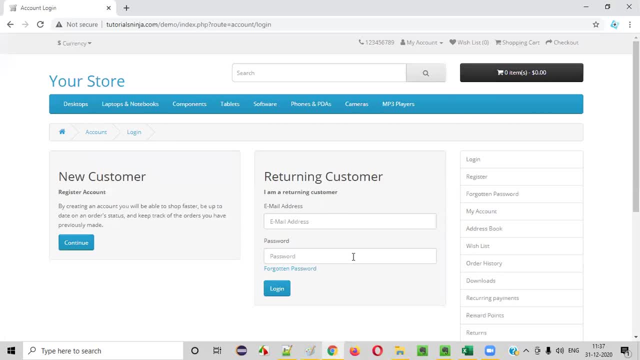 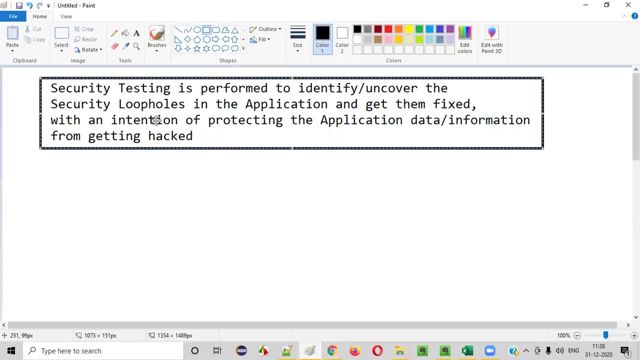 application. rather, we will check whether this login functionality is secured or not. that's what is secure testing will do so here. if you take this example- guys, login login example- and compare with this definition, you will understand more about what is secure testing in a better way. secure testing is performed to identify or uncover the security loopholes in the application. let's 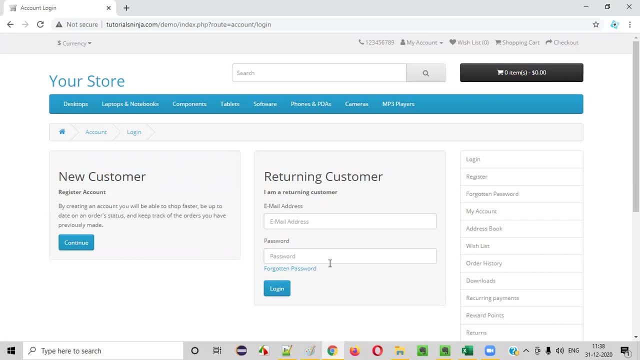 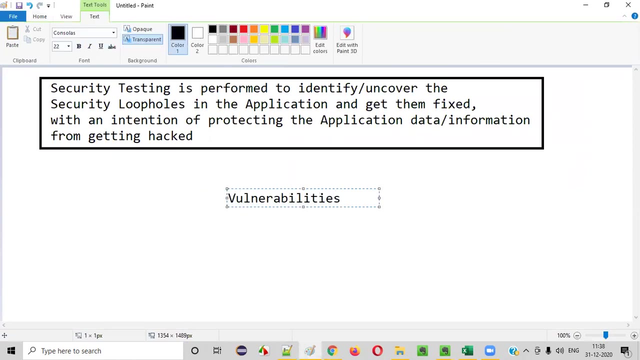 say, you are testing this login functionality. while testing this as part of secure testing, you will check whether this login functionality has any security loopholes. okay, so we generally call the security loopholes- as terminology, wise guys, vulnerabilities. in the security testing point of view, you call this security loopholes, security loopholes as vulnerabilities guys. so 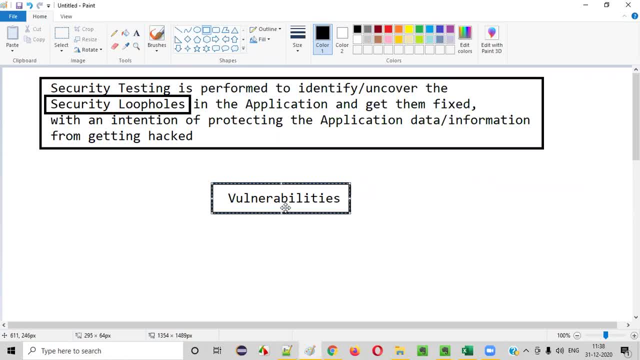 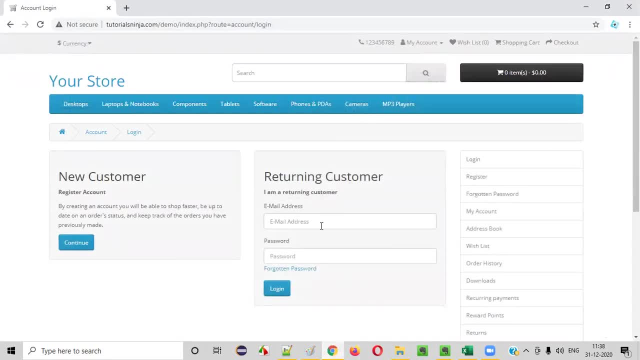 you have to perform security testing with an intention of identifying the vulnerabilities in the application, that is, security loopholes in the application. you have to perform security testing with an intention of identifying the vulnerabilities in the application. does this login functionality has any loopholes, security loopholes or? 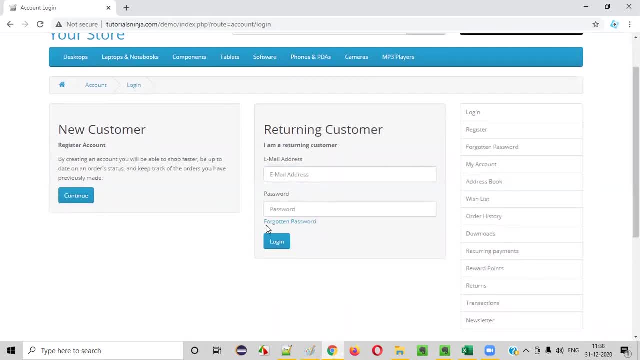 vulnerabilities using which the hacker can log into the application even though he doesn't have any credentials with him. okay, one example i am giving guys. let's say this login functionality is there and, because of because of some security loophole or security vulnerability in this login functionality of this application, hacker is able to log in into this or log in to your